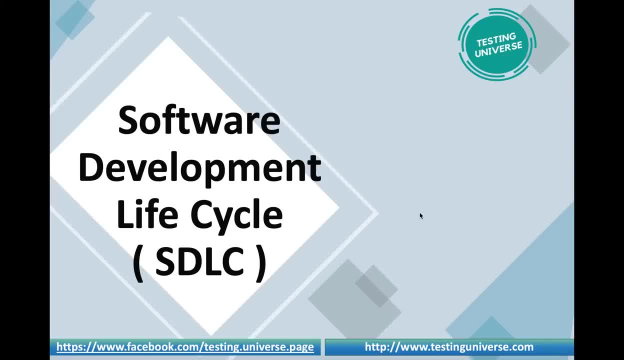 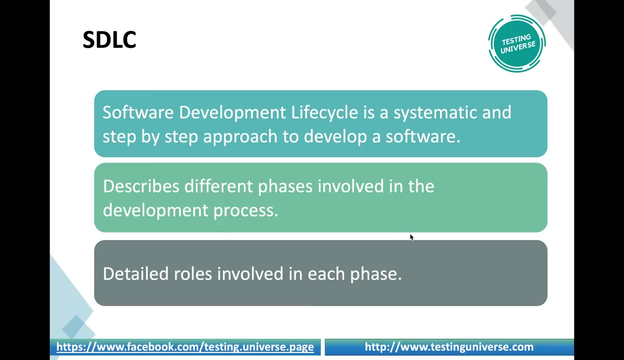 any software. software development lifecycle is an approach we have to follow, right? so what exactly is this particular software development lifecycle? how exactly it will guide us, you know, in developing a software. we'll try to understand everything in detail about this. so what is software development lifecycle? it's a systematic and step-by-step approach to develop a 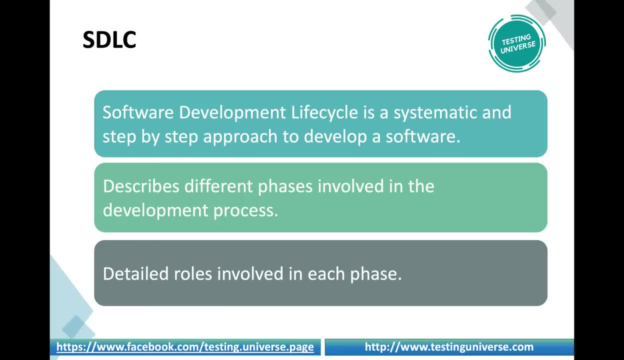 software. you will be having a systematic as well as different steps will be there right with that approach, we are going to develop a software. so software development lifecycle. it describes different phases involved in the development process. if you want to develop anything right, you will be having. you are, you will be you. 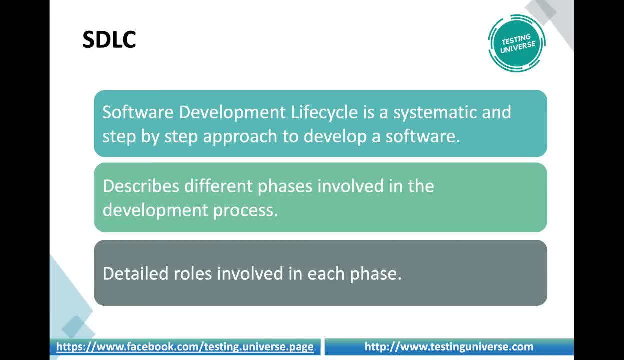 know, dividing that particular entire development into different phases, right, are different steps we can consider for now, right, once we go in detail about this, you will understand about what are these different phases. it describes different you know steps involved in the development process and it also, you know, gives the detailed roles involved in each phase means okay. 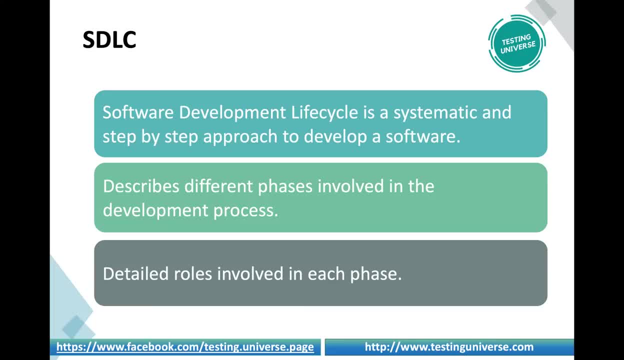 step one. I'm doing something in that what all roles- roles in the sense, what are, which are persons, which are you know involved, and what are those that person roles right it, this entire software development lifecycle will give you a detailed overview of how exactly you know you're going to approach to develop a 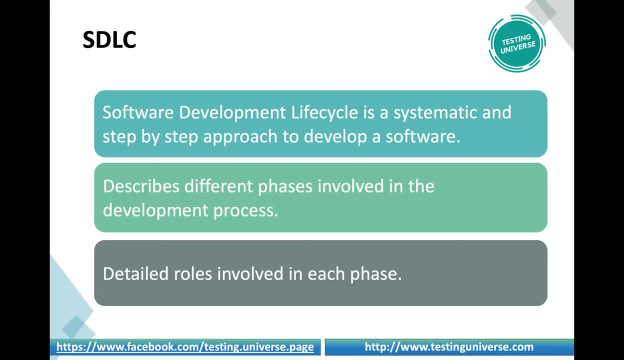 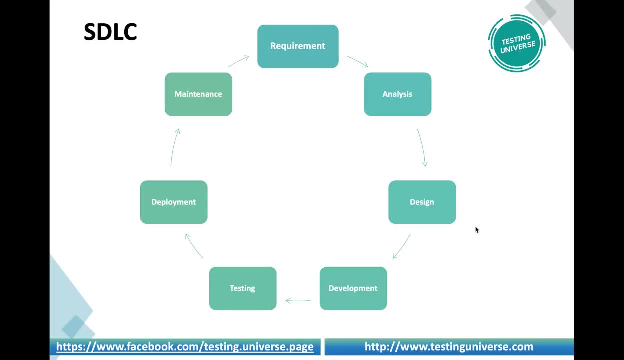 software and then we're all involved in that particular. you know approach, right, so we'll go ahead and understand right. what are those phases? right, you can see here in this diagram these are the different phases which are involved in developing a software. so what are these phases? the first phase is requirement. 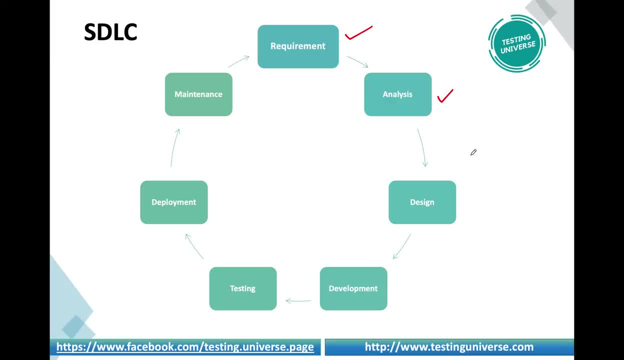 phase. the second phase is analysis phase, third phase is design phase, fourth phase is the development phase, fifth phase is testing, sixth phase is deployment and then seventh phase is maintenance. okay, we'll understand about all these phases in detail, right, but you can see here what is this requirement? we have to go. 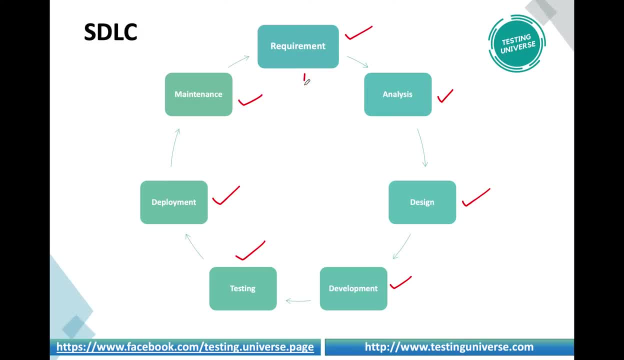 in detail about this and this is one phase or one step right, and then we're all involved right in this particular phase. so, before we go in detail and understand like how exactly you know we are going to approach all these different phases, we will take a day-to-day activity which will be 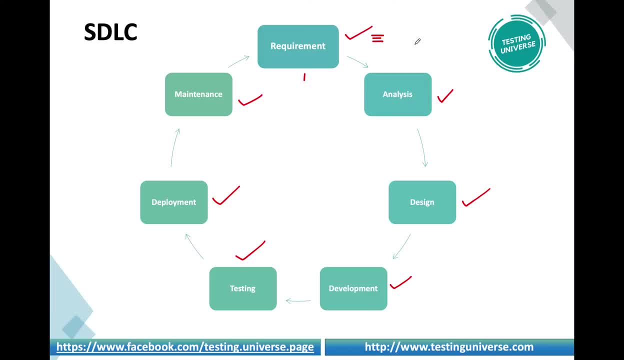 done by most of the human beings. right, just to give a broader picture or just to give a overview of how exactly you know it is. it has similarities to develop a software. i'm going to, you know, take an example of right: constructing a house or constructing an apartment or anything, right. 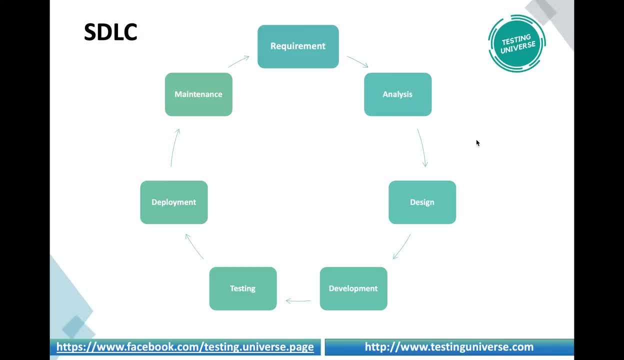 so we will take up that example. that's a generic example i'm going to take so that you will understand. you will understand what exactly you know a person will do while constructing a house. so similarly, we will apply the same rules in software development, right? so if i, if i want, 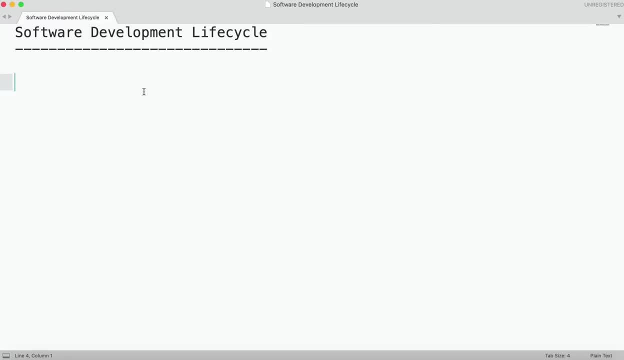 to construct a house. okay, let me, let me just go in detail about this. right, i want to, you know, construct a house. so i will be having certain requirements, my own requirements to construct a house, right, so what are those requirements first? first, i will, you know, tell i need, i want to construct a house with three bedrooms. 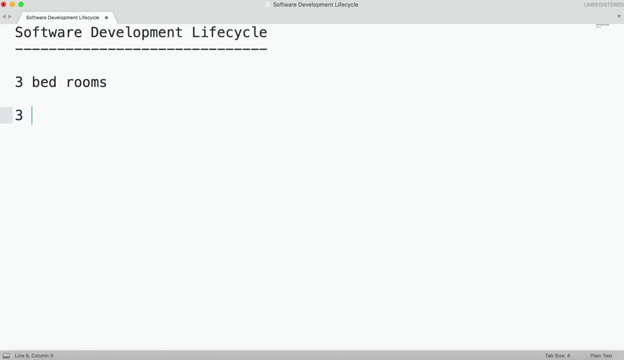 and three bathrooms and i want to have a nice right garden in front and whatever these three bedroom, this house should be a duplex house, okay, and i need to have a nice garden. i need a- you know- car parking space for two cars. okay, we can, we can consider it as big cars. 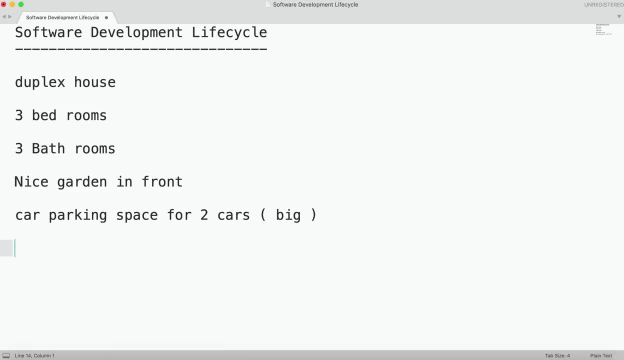 two big cars and then i need, i want to have a parking space for two bikes. just just, you know, there might be a number of requirements. i'm just, you know, giving you with these requirements. we're giving you an overview, okay, so let's, let's, you know. 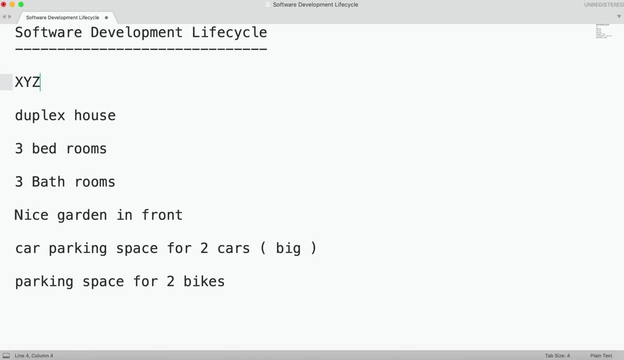 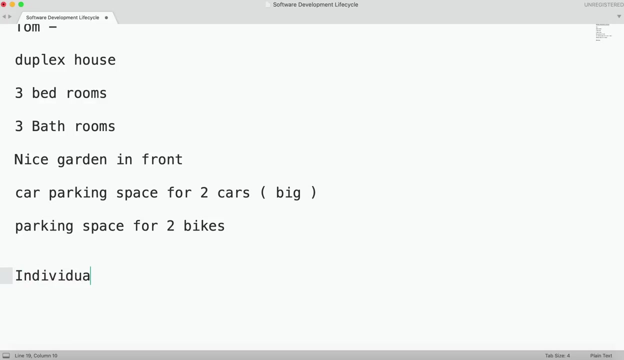 consider a person by name xyz right, or we can. we can also take it. take him as tom right. tom wants to construct a house with these requirements. so what he will do, he will either approach an individual- you know a builder- he might approach an individual builder- or a company. he might approach an individual builder or a company. 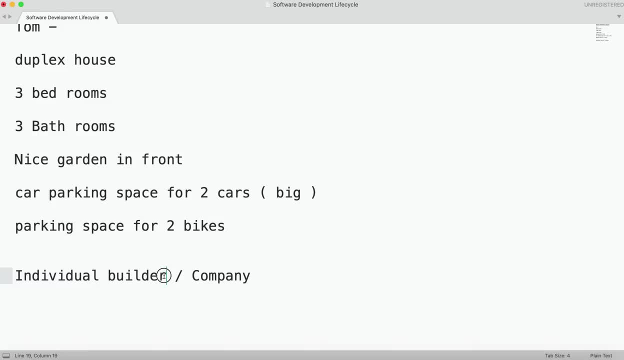 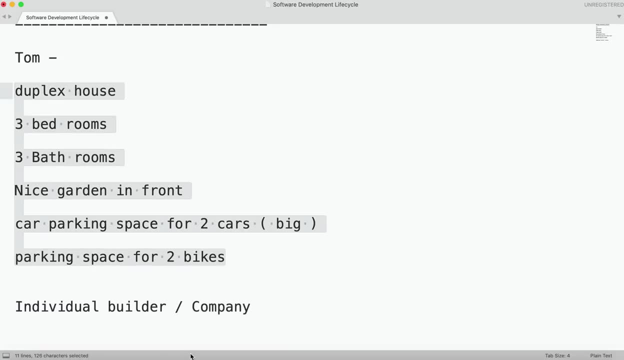 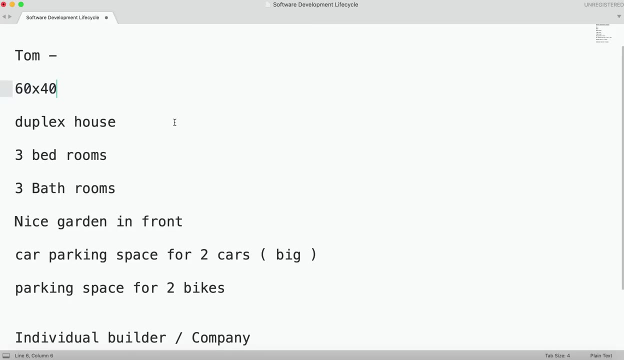 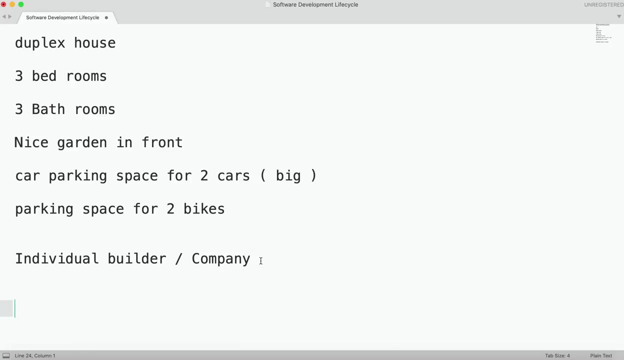 okay, let's say he has, he has approached a company right. and then he will say: right, these are my requirements. i want to construct my house. i have a plot of 60 by 40 right in this. i want to construct a duplex house with all these requirements. okay, so this is called a requirement phase. means tom tom, if you consider. 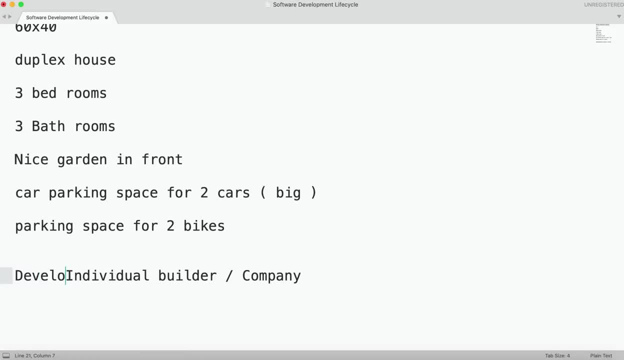 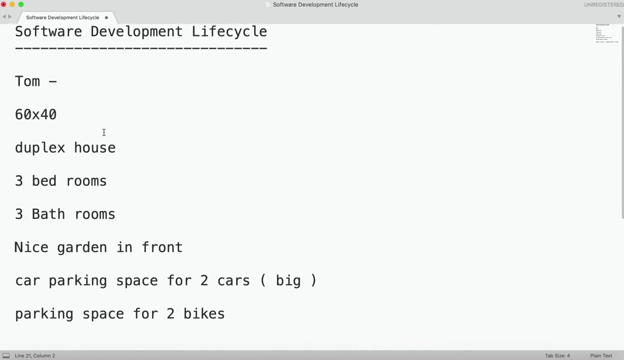 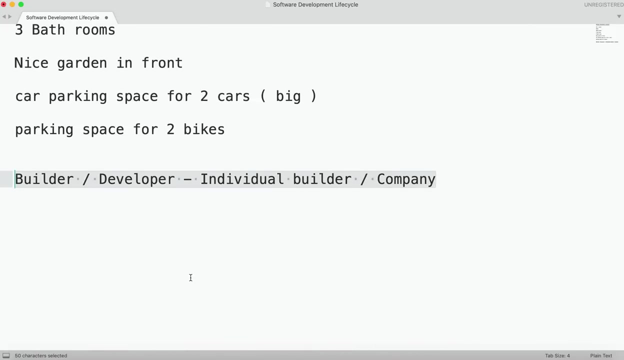 the company. this company or individual will be a developer, okay, or a construct construction company, or you can consider them as a builder or developer. okay, you can consider them as a builder or developer and this particular term will be a client to these builder or developer. it will be a client to this builder or developer. so. 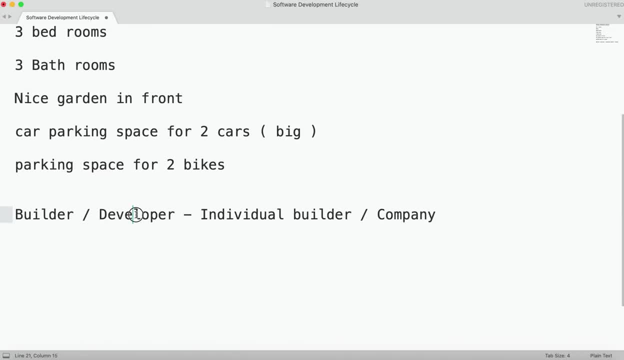 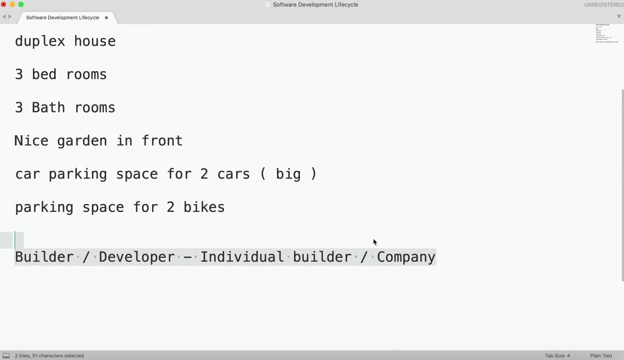 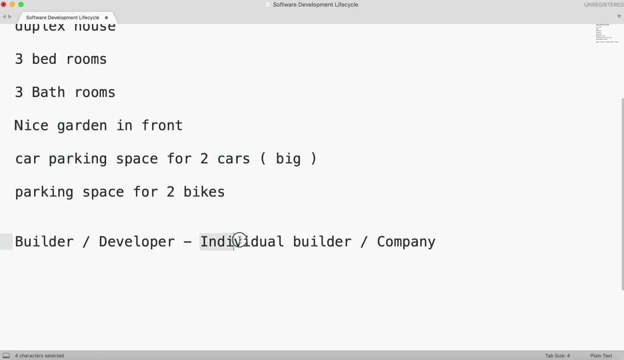 the client is going to approach the developer or the development company or the builder company to develop a house with all these requirements. okay, he will give the requirements so from from this company or from, uh, if he is an individual builder, any, any one person, okay, will be assigned. 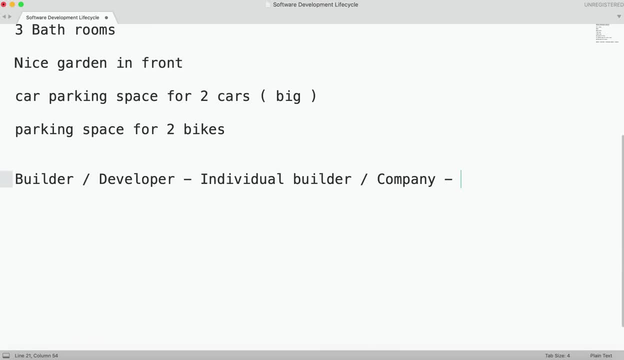 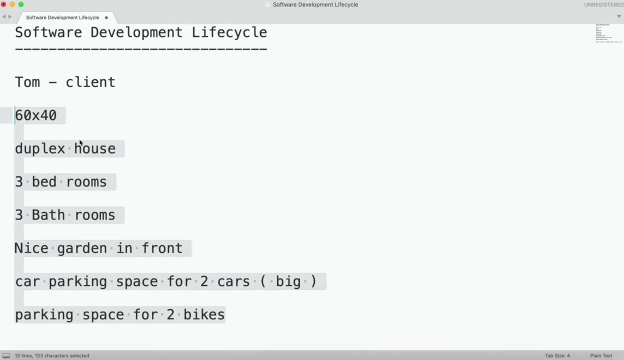 and that person, for example, by name henry. okay, he's going to gather the requirements, he's going to take all the requirements of the tom, and then what he will do, he will analyze all these requirements. okay, okay, tom, i can- uh, you know- come up with some design for you. i can come up with some design for. 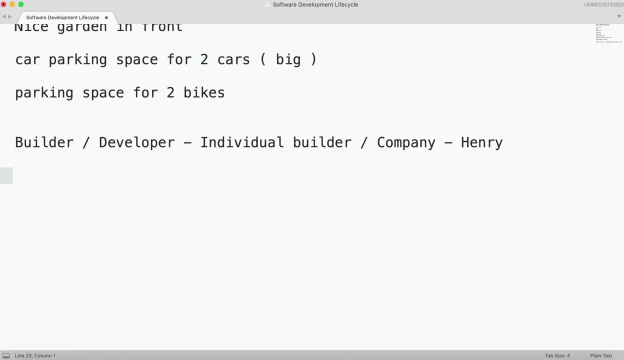 you. so he will what he will do. since they're- they're from the builder company, they're going to give the design. how exactly the design would be. the design would be like: uh, the architecture. right, the design would be the architecture or the you know high level. 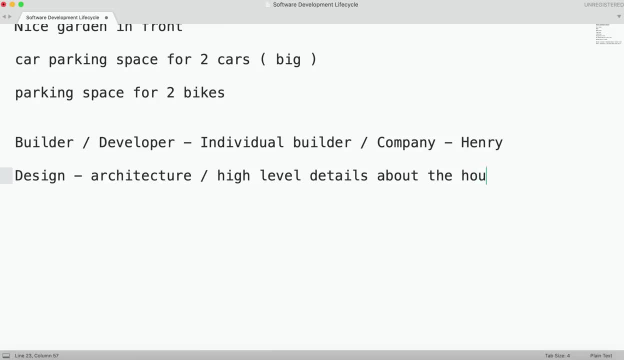 high level details about the house, which means they will give a diagram in such a way that, okay, the entrance will come here, the you know sit out will come here, the hall will come here, like that, a bigger picture they will give. along with that, they will, you know, give you a 3d. 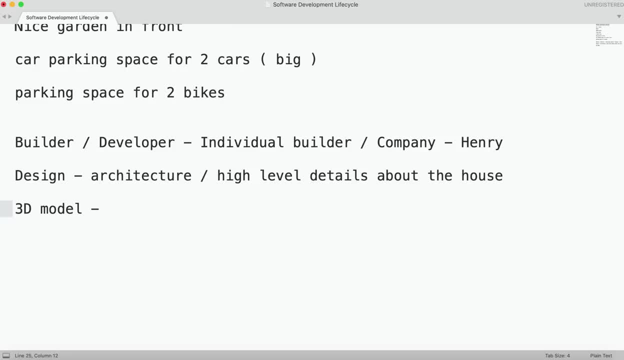 model, which is the detailed design, which is a detailed design. what is this detailed design? okay, in the hall, what all you know minute details will be there. that level of detailing will be given in this particular 3d model. okay, so this is called. this is called right, low level or 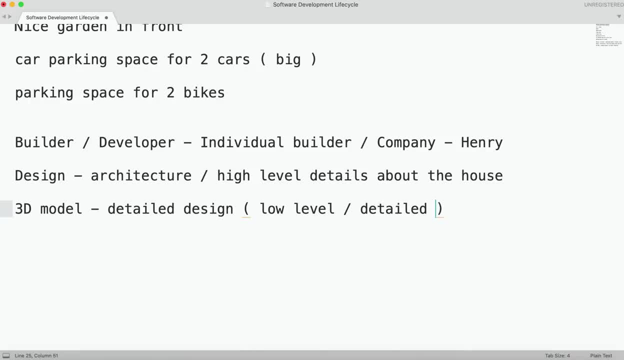 detailed design is called low level, or details means in detail, everything will be explained in this is: this is a high level architecture. okay, this is how it looks, and then it will be given in this particular 3d model. okay, so this is called low level or detailed. 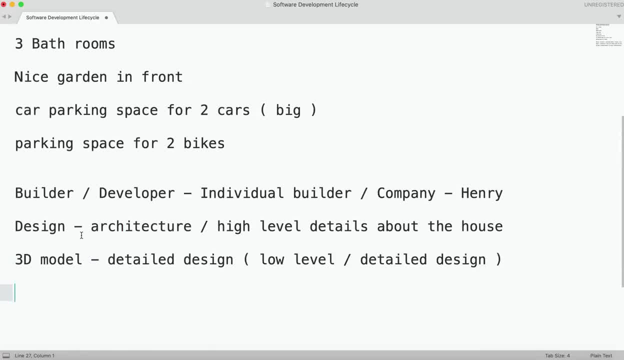 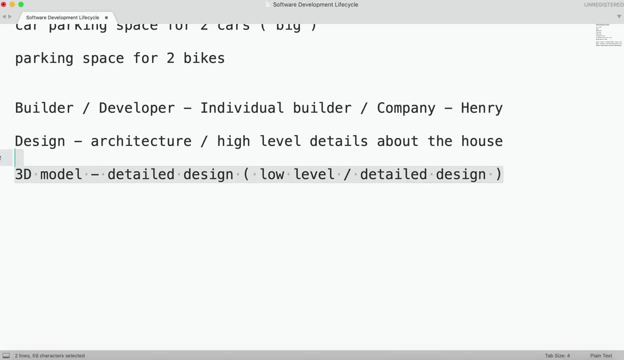 detail, each and every you know room, each and every requirement will be considered. so, after, after, you know, giving all these design, if, if you are okay with the design, you will tell the company: right, okay, I am okay with the design, let's start building the house. otherwise, if you need any modifications, you will say. 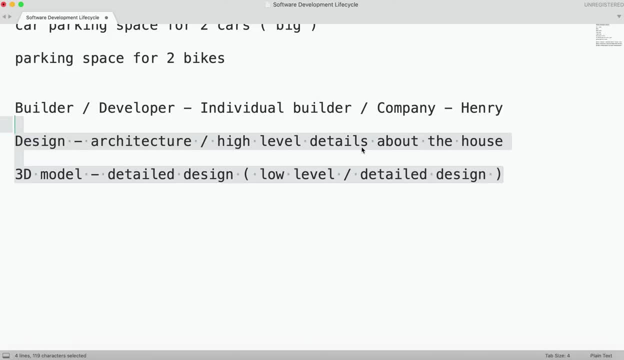 no, no, no, I need some changes in this particular you know design so you can make those changes so that we can go ahead with the construction. so let's say you, you have, you know, come to an agreement. okay, I am, I'm okay with this particular design, let's, you know, start the construction. so the the Henry's role. 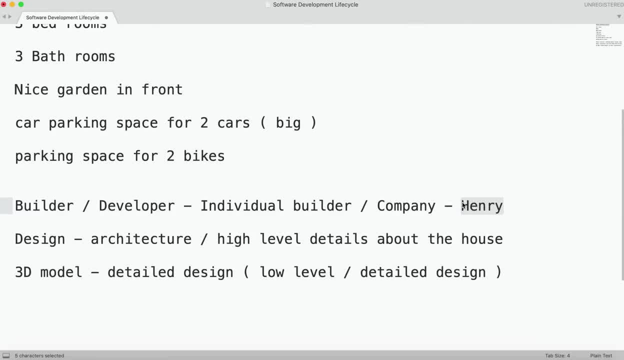 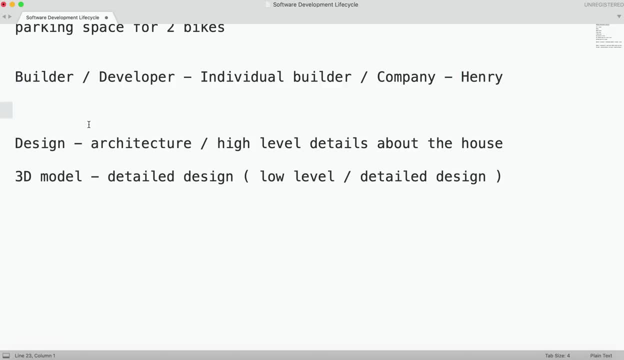 gathering, the requirement will be over. once Henry gathers the requirement, the design and everything will be done by some other person. okay, there will be a separate team for designing design team. they will give you the design. design team will give you the design one that is done. there will be a different set of people right to 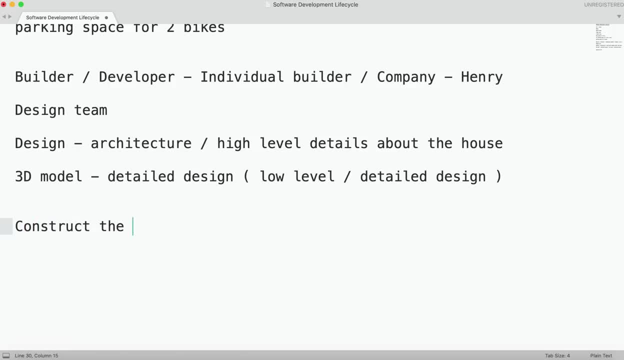 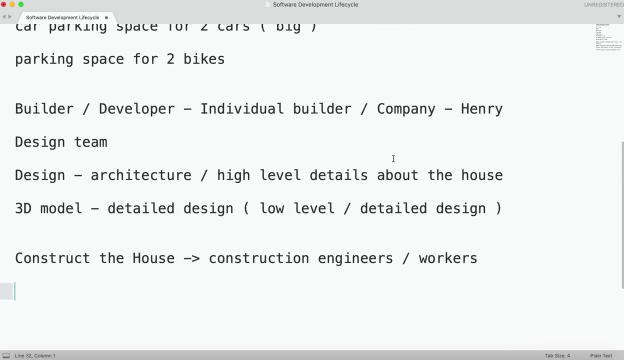 construct the house? okay, to construct the house, different set of people will be there. okay, construction engineers and workers, let's take this right. so as soon as they start the construction, right, there will be a lot of agreements. okay, this, this is the pricing, and all those details will be considered. and then, once everything is, 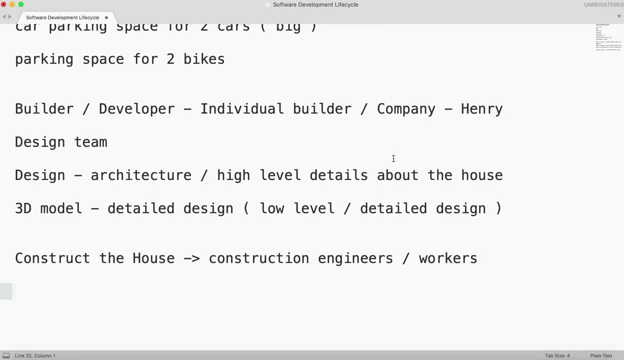 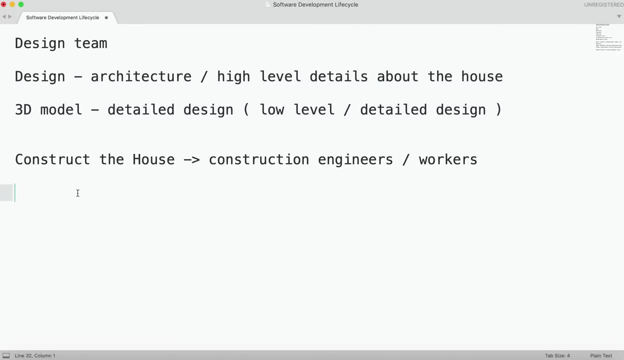 agreed, the no construction of the house will start. and then, once the construction starts, okay, at the design phase you might be having some certain you know ideas, but when the construction of the house starts you might, you know, as, as and when the progress goes, you might come up with 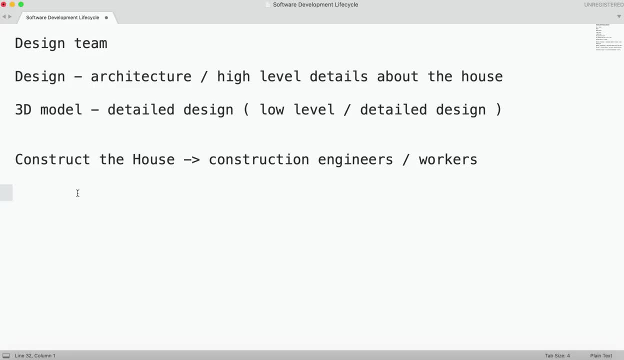 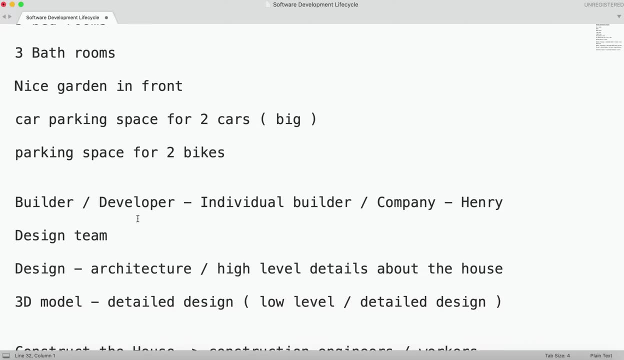 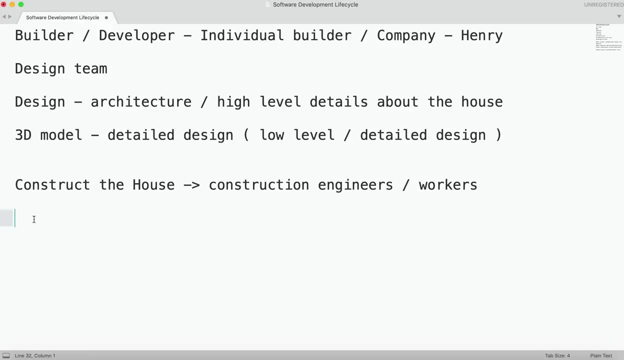 different ideas. also, if there is an agreement between you know the client and the company right or the developer, then only there they're going to allow the changes. otherwise, as for the design, the construction will happen. once the construction is complete, it will be handed over to the. it will be handed over. 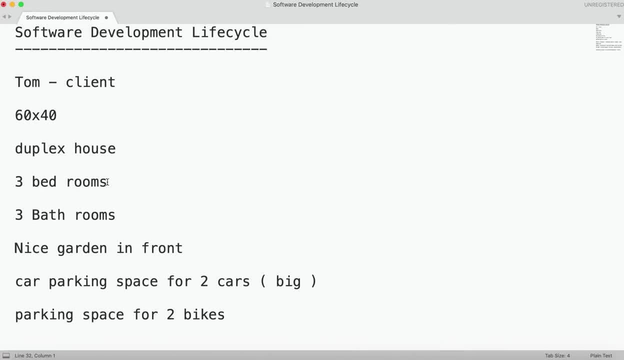 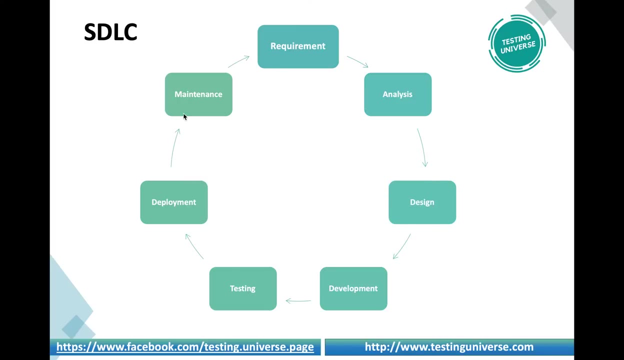 work to the client, right? so that's how we are going to construct a house means if i want to construct a house, also, i am following a step-by-step approach in a. in a similar fashion, if i want to develop any software, we have to follow a step-by-step approach to develop a software. so what? 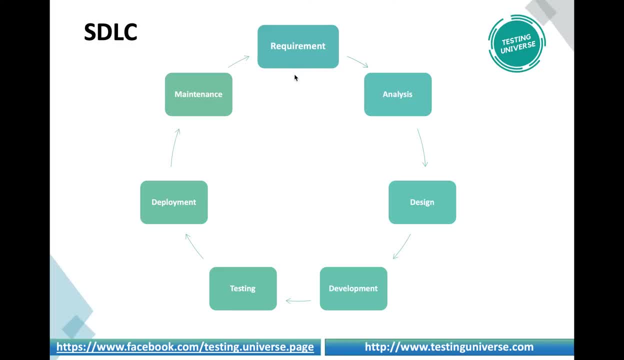 exactly will happen in each and you try to, you know, analyze whatever i have given as an example for the construction company, because that that will remain that in a in your day-to-day life, you will be doing or you will be seeing all those activities and you can compare the same thing. 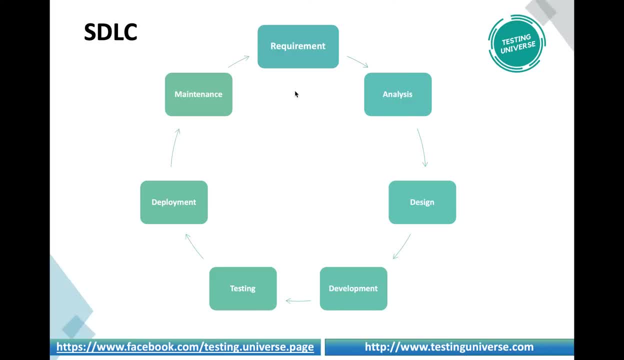 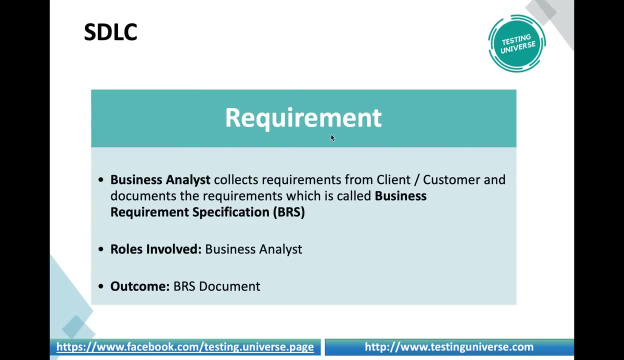 with these particular requirements. okay, so let's understand everything in detail about this particular software development life cycle. the first phase is requirement phase. in this phase, what happens? business analyst collects requirements from client or customer and documents the requirement, which is called business requirement specification document. okay, the role. 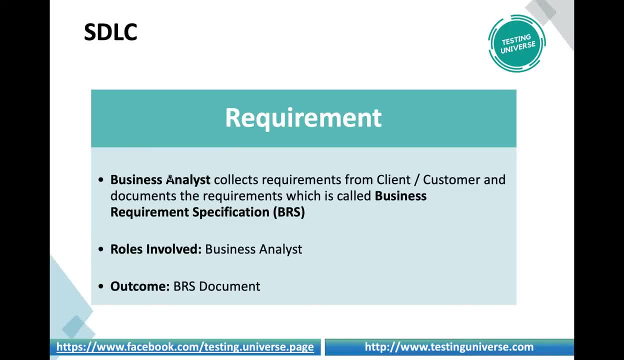 is business analyst. the business analyst from from the you know development company will sit with the client or customer. there will be an individual or maybe group of people from the customer end and the business analyst will meet together and then the client will explain all his requirements to the business analyst and then, after 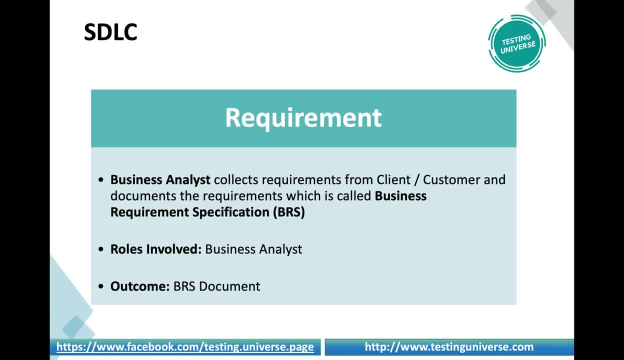 you know, collecting all the requirements of the client, business analyst will create a document which is called business requirement specification document, which is brs, or it can also be called as customer requirement specification document. right, so that is the requirement phase. so what, what client will do in this particular phase? right, we will take an example of a real world software application. 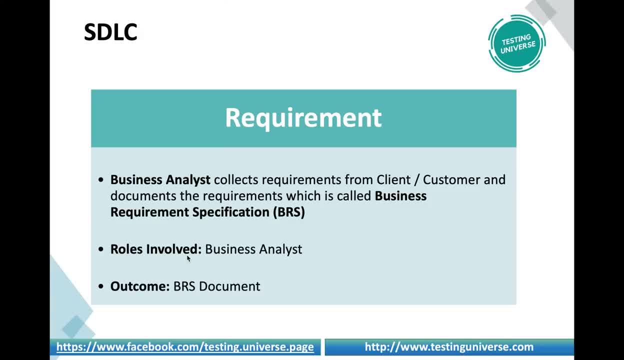 and then we try to understand that. okay, So the role involved in this particular phase is business analyst and the outcome of this particular phase is business requirement specification document. Okay, So that's about the requirement phase. So what is the? what are these requirements? right? 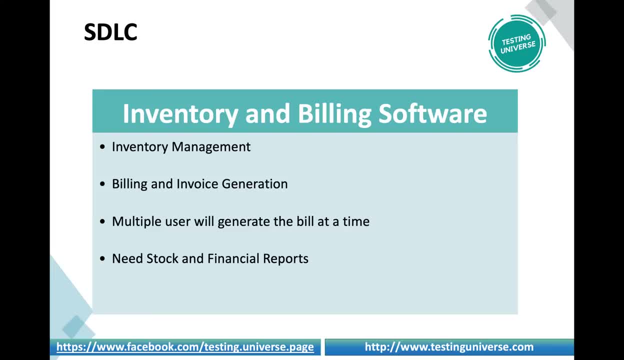 Let's take one example of inventory and billing software. right, In this particular. what is this inventory and billing software? I will. for example, I am a company who sells mobile phones. right, I want to maintain my stock and then, whenever a phone is sold, whenever a phone is sold, 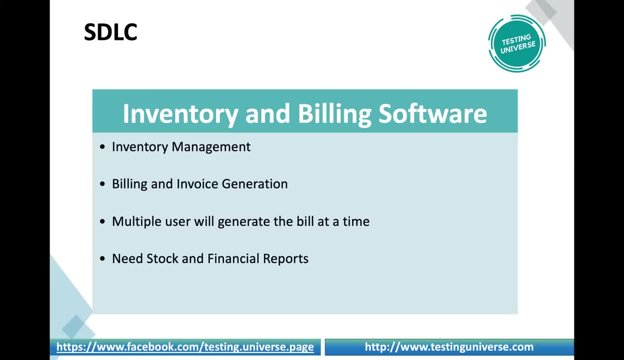 I have to build that particular customer who is buying it, and then my inventory or stock should be reduced. That kind of you know it's a billing software, which is also called as point of sale software, which is very common. you know, you will commonly, you will see across. you know all the you. 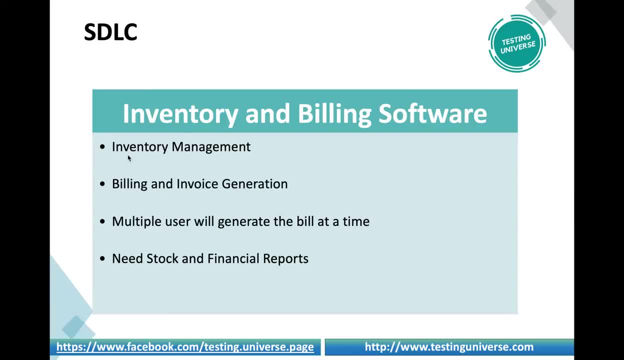 know industries right. So what is this? What is this? In this the client will say: I mean, I want to maintain my inventory, I want to, you know, build and generate the invoice to the customer, And then not only one user, multiple users will generate the bill at a time. 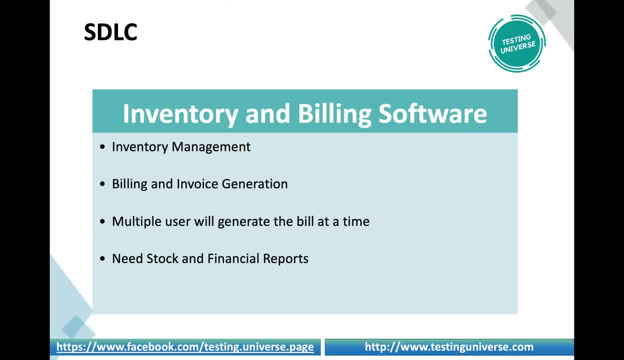 For example, if you go to any shopping mall or if you go to go to supermarket, there will not be only one counter, but multiple billing counters will be there, But the software There is one, each and every billing counter. one person will be sitting and he will be. 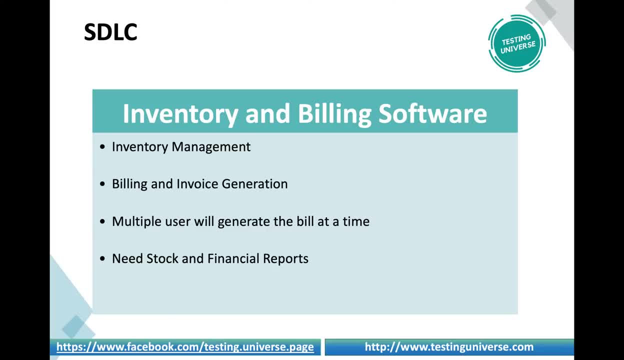 having separate, you know, login, separate username and password to that particular software to bill, right. So that's the requirement and need. stock and financial reports means stock means okay, how many are sold, How many are available in my inventory or in my go down? 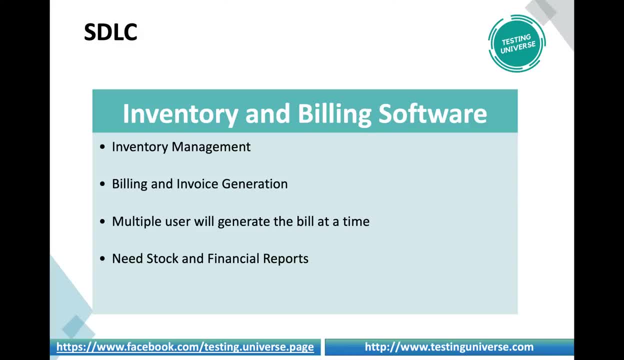 And then how many? you know today how much money I have generated. or it might be a daily basis, It might be a monthly basis or yearly basis. Whatever date the customer selects, you should be able to generate the financial reports. 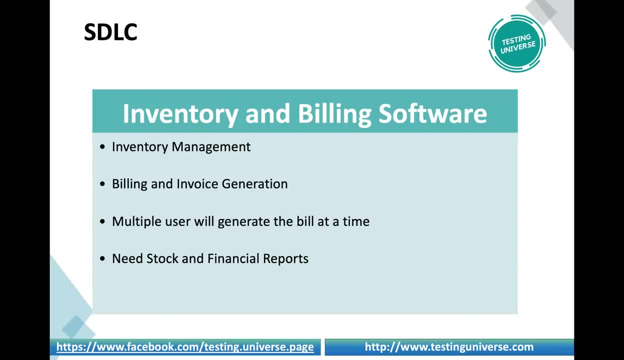 also Okay. So this is the requirement is given by the customer, uh, uh to the business analyst. Okay, We'll, we'll go in each and every phase. We will take this inventory and billing software and we'll try to analyze right. 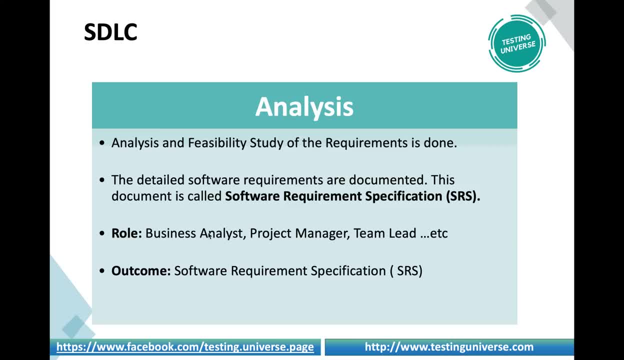 How exactly you know a software will be built. The next phase is analysis phase. Okay, The requirement is given by the client. but whether it is feasible to develop all the requirements given by the customer or client or not, that analysis will be done. 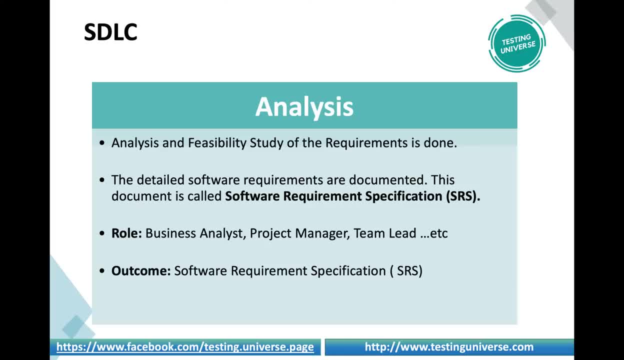 Okay, Analysis and feasibility study of the requirement is done. Not every requirement will be, you know, converted into a software. There will be. there will be, uh, you know, some restrictions also, right, While developing the software. Okay. 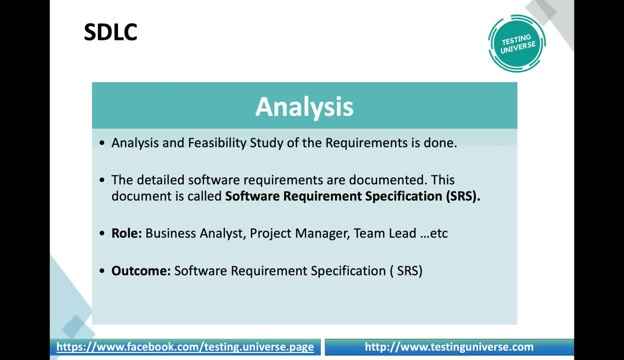 So the customer on his day to day basis, whatever he does uh in his uh you know a store or in a supermarket or wherever it is, he's going to explain that to the business analyst. but not all the you know uh requirements, uh, uh can be uh we can always fulfill all the requirements or there might be some uh restrictions in fulfilling all the requirements. 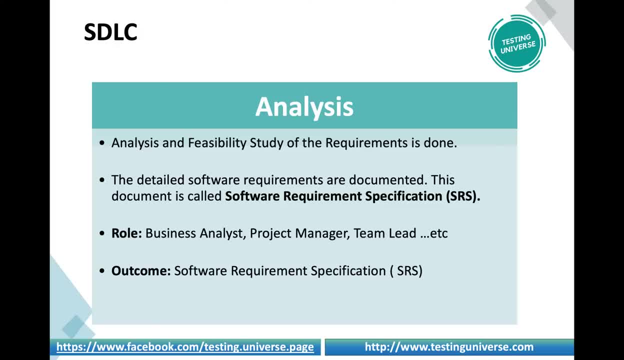 So we have to do a feasibility study of all the requirements, Right, And we have to analyze the requirement and we have to do feasibility study of the requirement. once that is done, So who are all going to, you know, do this particular, uh, feasibility study? 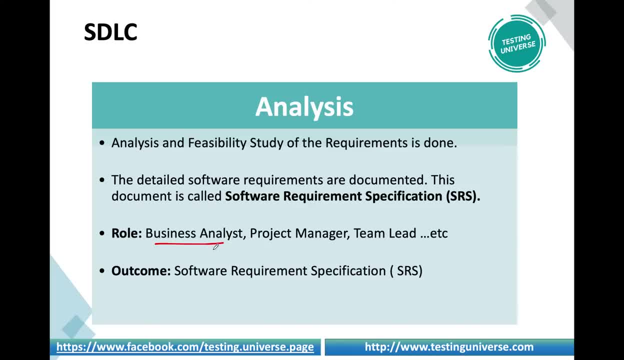 So you can see here business analyst, because he's the person who has, uh, who, who is interacting with the customer. So, business analyst, and then the project managers, right? So these, these people are uh, uh, you know, from the development team. 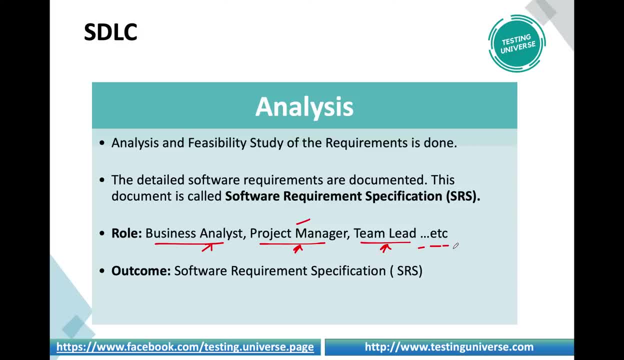 Okay, And then different team leads and it, it all depends on the company, But these are the main- uh, you know- roles which will always be involved in analyzing the requirements. once they analyze the requirements, So they will, they will filter out. 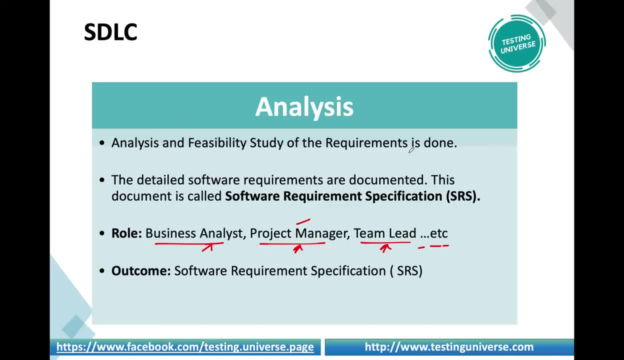 Okay, I can, I can, we can develop this particular software for these requirements, Right? Uh, a detailed software requirement are documented. So, whatever already, uh, the requirements given by the client, it is it, it will. it will not be, you know properly, you know, designed to develop a software. so there will be. 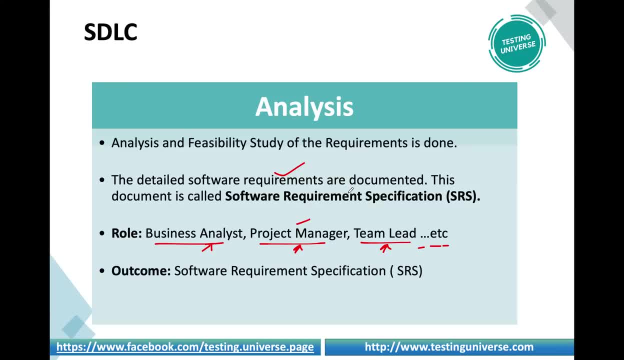 a document which which is generated, which is called software requirement specification document by these people, right? so, in this phase, what happens? we are going to write a software requirement specification document, along with analyzing the and doing the feasibility study of the requirement. so the outcome is software requirement specification. 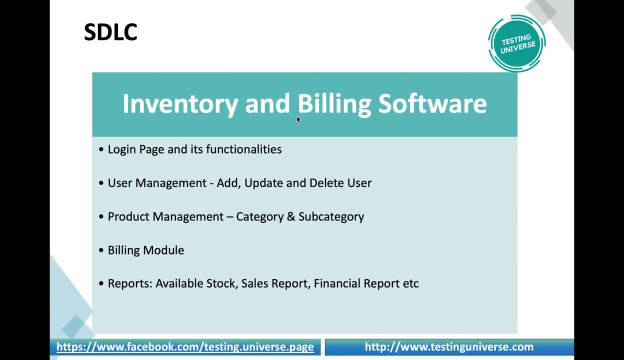 document. so what is this software you can see here? this is how the software requirement specification- uh, you know uh will be uh- detailed out for a billing software. let's say, i want to have a login page and its functionalities like username, password needs to be entered if wrong. 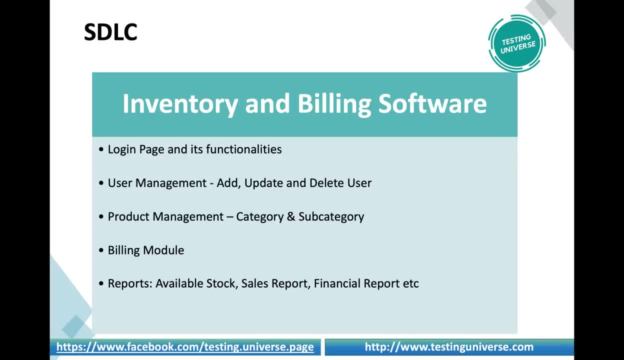 password is entered, you know you need to show the error message. all those detailing will be written there. and then customer told multiple users: uh, you know, needs to log in and build the software. so we need to have a module. we can we call you know these things as modules, right, user management. we need to have 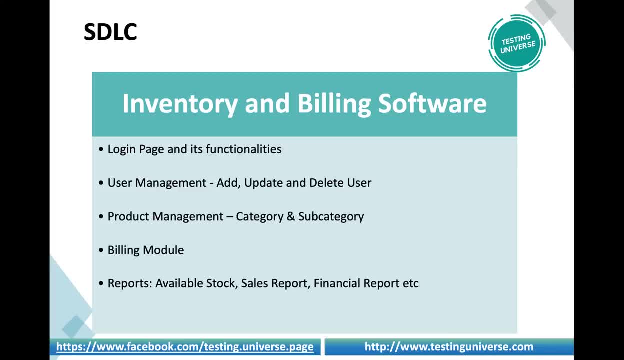 user management like: add user, update user, delete user. if they leave the company, they have to delete the user right. update the user if, if they have entered wrong data, they want to update the user right. while while adding the user, you need to create their username, password and all those. 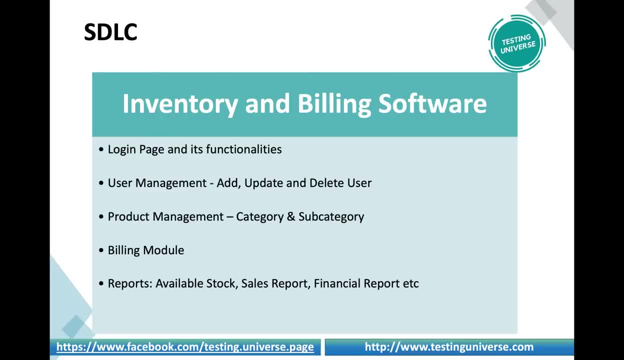 things. all these detailing were not given by the client in the requirement phase, right. so these kind of detailing uh will be written by the written in the software requirement specification document. so, similarly, product management: right in the product management you will be having category and subcategory. right in the in the smartphones you might be having uh, you know, in the phone. 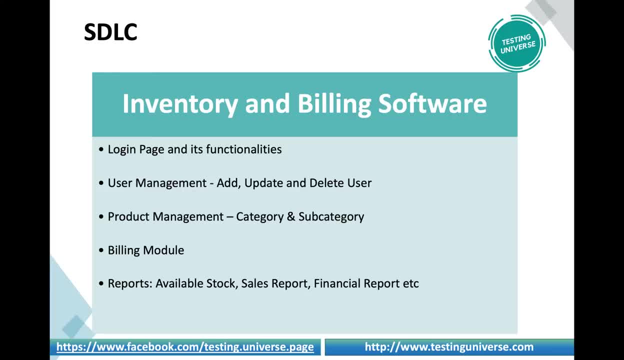 industry. you might be having smartphone, normal phone, like that. different categories will be there and then different companies will also needs to be added right. like that, you need to have product management module and then billing model and then reports module. like this, everything will be, you know, written. 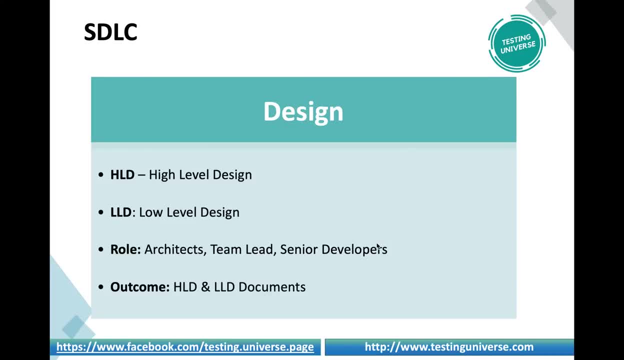 in detail. right, that's about, uh, the analysis phase. once the analysis of the entire requirements are done and once software requirement specification document is generated, they will once again, you know, sit with the customer and then they will give the detailing about it. okay, this is how, uh, you know, the software requirements will be filtered out. these are: 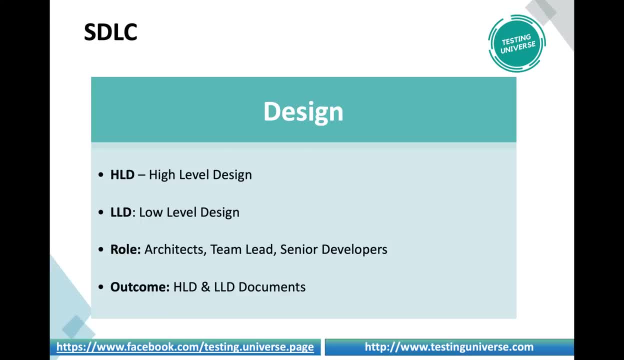 the software requirements we can develop. and these are the requirements we will not be able to develop. okay, so they will. they will sit in detail and then they will come to an actual agreement. okay, this is fine. you can go ahead and give me a design like how exactly? uh, you know, the software will. 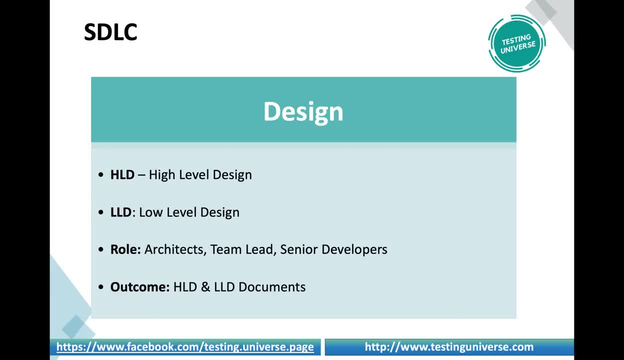 will look on a high level and then give me a detailing about it and start developing the software. so in the design phase there are two uh types of design. one is high level design and low level design. you can, you can see here the similarities, the same thing you, if you go back and 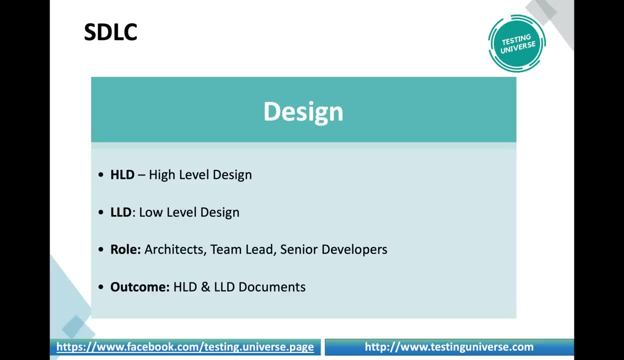 do the construction, the. there is a high level design which which will be given uh by the company and then did in detail about each and everything will also be, you know, charted out right. so similarly, in software also, we will be having high level design and then low level design. what is this? 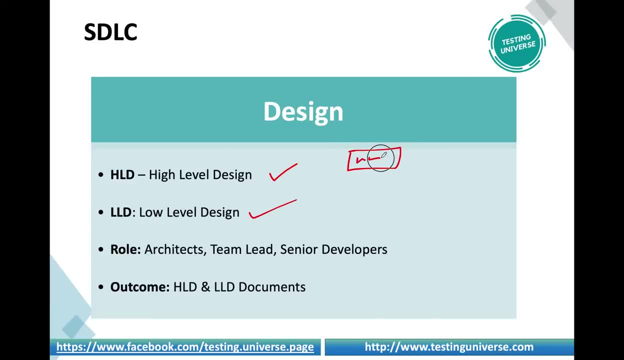 high level design. okay, i will be having, uh, you know, user management module. like that, there will be some architecture with which will be, you know, uh, charted out, there will be, okay, this is the flow and then, like that, the the high level architecture will be written. these are the modules will be there. 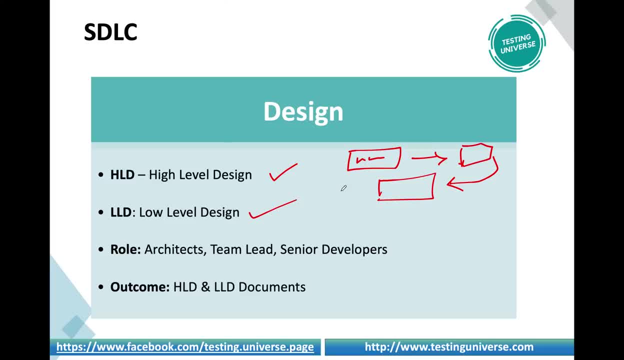 and then certain modules will interact each other like that, high level architecture will be given. that is high level design, and in each and every module you might be having sub modules also, right? so those things will all always been, you know, considered in low level design. those things will always be considered in low level design, okay, or uh, detailed design. we. 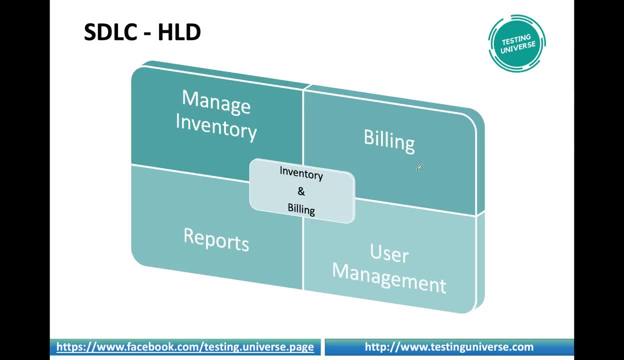 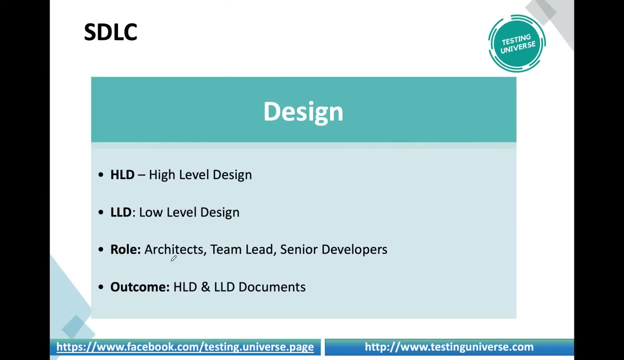 will come to this. we'll take up an example of that you know, inventory and building software- and then we will, uh, you know, understand this. so what, overall, uh, you know, will be involved in this? the developed architect, architect from the development company? okay, this, this person is the main person who is going to, you know. 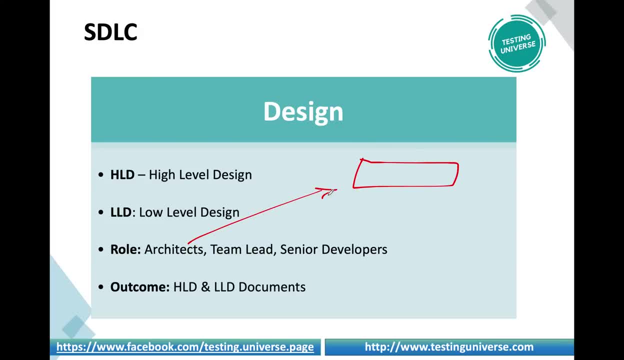 with the help of software requirement specification as well as business requirement specification document, he is going to right uh give the high level and low level design documents. so, along with him, team leader and senior developers will also be involved in this. okay, so the outcome of this particular uh? 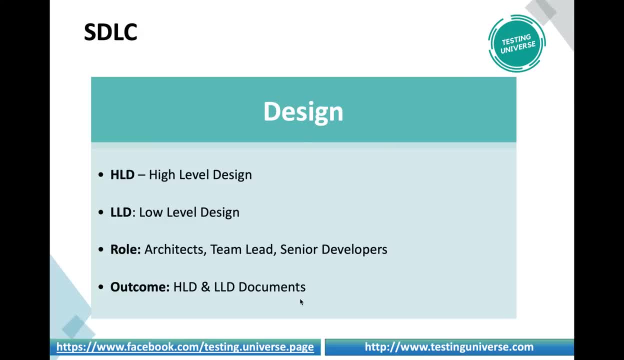 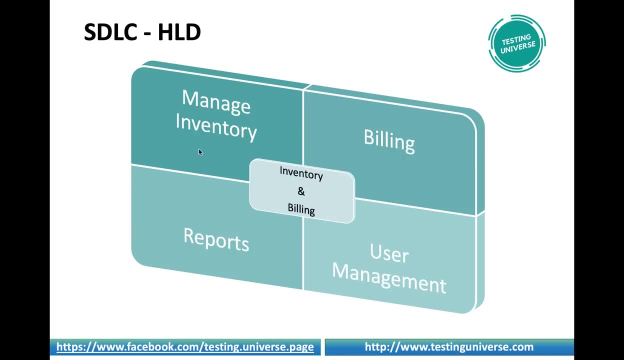 phase is high level and the low level design documents right. so we'll take up the same example you can see here: inventory and building software. the high level architecture would be manage, inventory, billing, user management reports, like this: a big module list will be given and then how exactly. 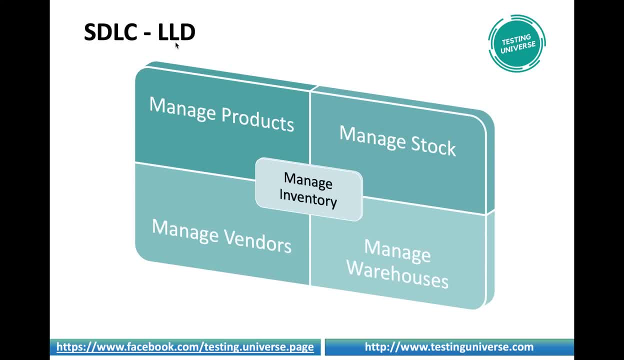 they interact with each other when you go to the low level, design, right. so in manage inventory, manage products will be there. manage stocks will be there. manage vendors will be there. manage where a process will be there, all right. so the detailing- uh, you know, will be filtered out, uh. 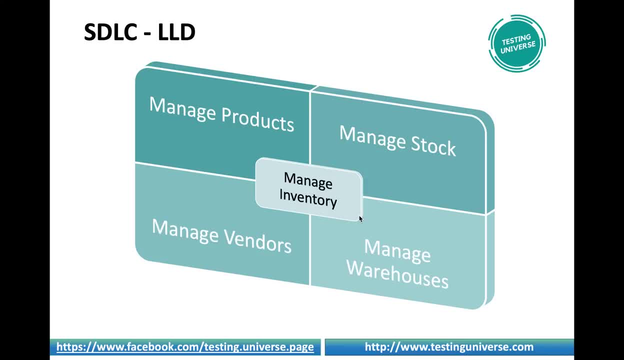 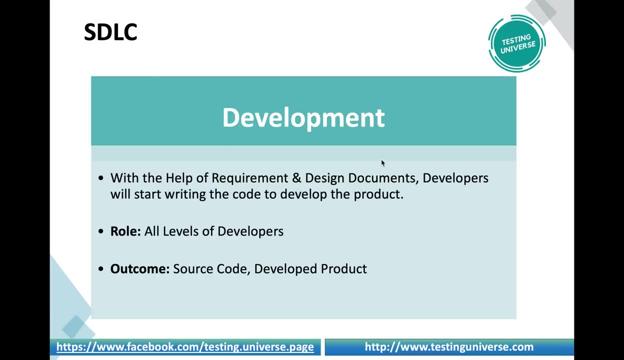 to the core right. that is low level design. that is low level design. that's about design phase. once the design is shown to the developer, okay, this is how the you know entire product works with sometimes what happens? they are going to develop this with some prototypes or some you know. 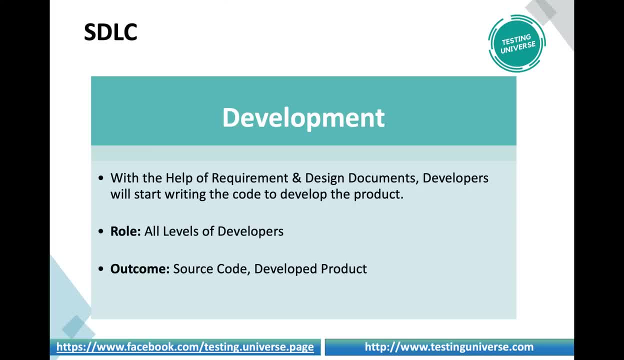 user interface, you will understand about all those things. what is the user's interface means there will not be any functionality, but you will be having, okay, a pictorial kind of representation will be given to the client. okay, this is how it looks, right, once the client accepts that. 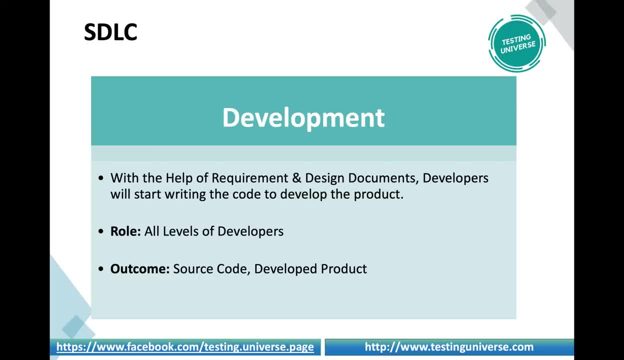 or if there are any changes he is going to, you know, suggest the changes or if, once he accepts that, the development phase will start. so, with the help of requirement, as well as the client's accessibility management, you need to write down what are the websites of the business. 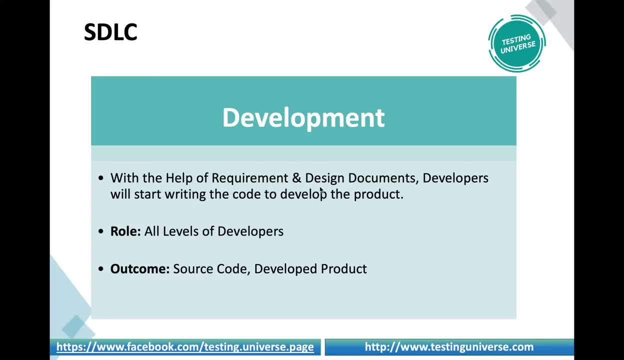 is that there is a lot of computer environment here in the development department, here in representation, as well as design documents developers. okay, the input for this particular development phase is requirement as coding languages or programming languages like C or C++ right or Java or Python, like these many programming languages are there. with the help of all these programming languages, 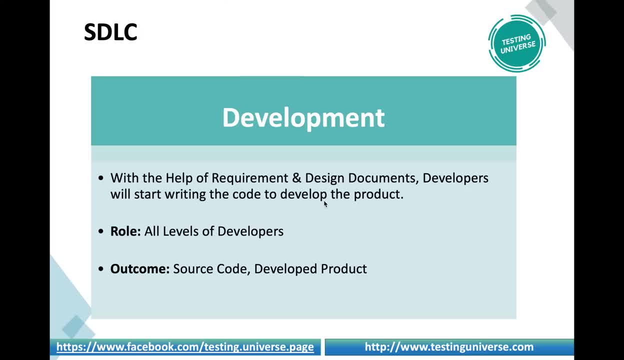 they are going to develop a software. it might be one programming language or it might be combination of many programming languages- right for a big enterprise application. it will always be a combination of multiple programming languages will be there. so all level of developers will be involved in this, in the sense the senior developers, junior developers and then 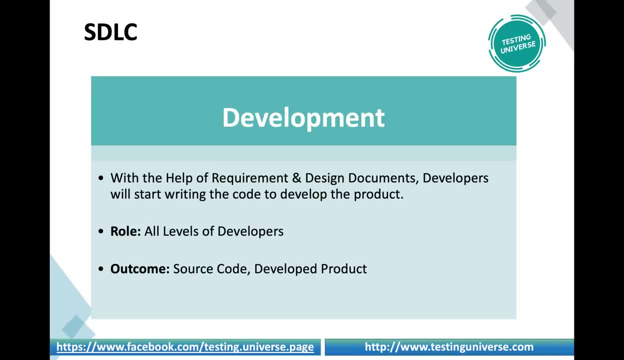 team leaders- sometimes team leaders may also- you know, code right- all those behind in the development phase, the project managers, also in, maybe you know- daily meeting or weekly meetings. they will be involved. so it is a it is a very, very big field- phase of software development. all those phases are, you know, one window and then this software. 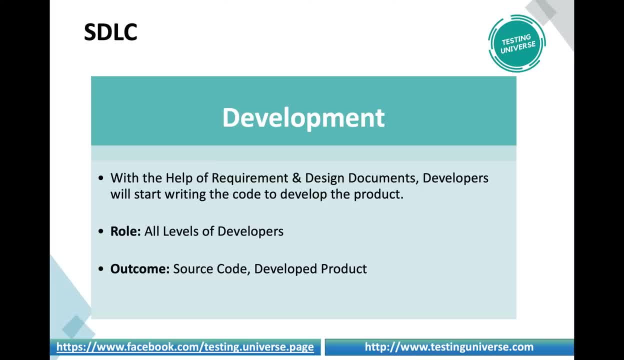 development is a very, very big phase because, whatever you have decided, you need to bring it, you know, as a software, bring the software as an output. so lot, of, lot of time will be, you know, involved. time and resources will be involved in this. so the outcome of this: 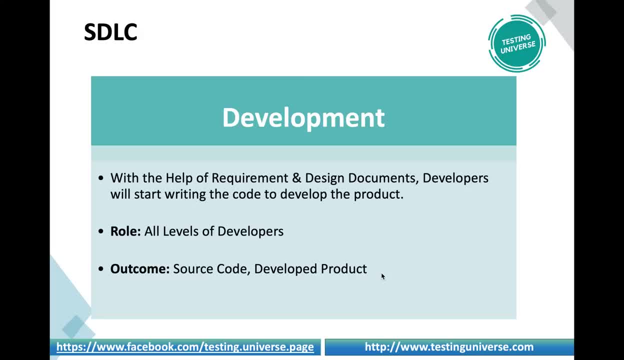 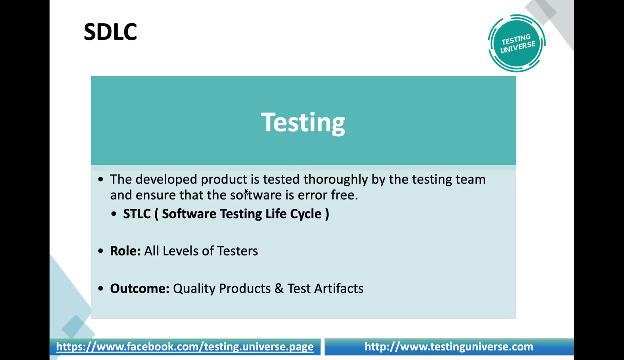 particular phase is source code as well as the software development phase. so this is code as well as developed product. so source code with source code in the sense where programming languages, whatever code you are going to write- that will be called as source code. and then the final. 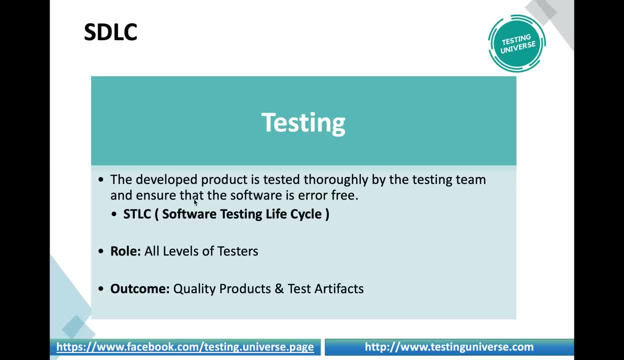 developed the product. once this particular phase is completed right, there will be a testing phase and accept and ensure that software is hasớv. so, like software, using software in need to be more useful for the application processum, to build up a protected set you development lifecycle, we also have software testing lifecycle. we will. 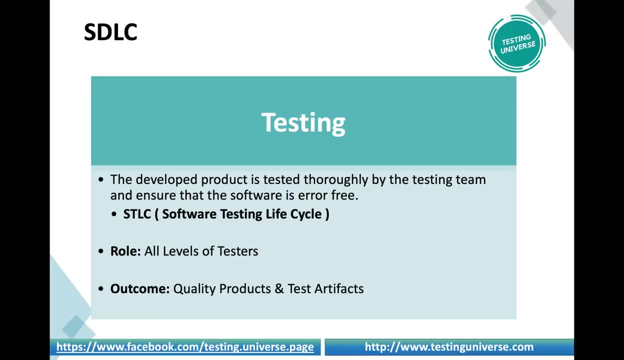 understand like what all the different phases which are involved in software testing lifecycle- even that is a, you know, testing is a part of software development lifecycle and in its own it has its own, you know, systematic approach and different methodologies will be there and different types of testing. 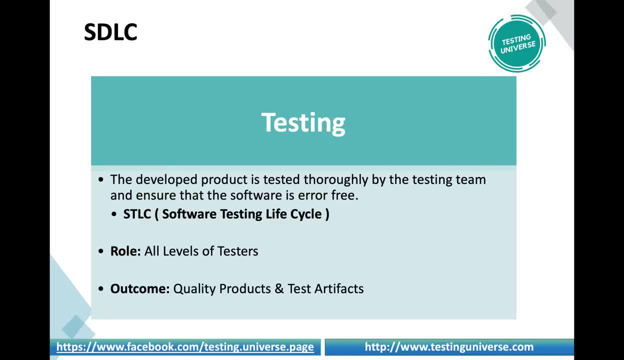 will be there. all those things should be considered while testing a software. so, with the help of software testing life cycle, the testing team is going to test the developed software. so what are overall rules which which are involved? all levels of testers mean Junior, senior testers, team leads, collect managers and 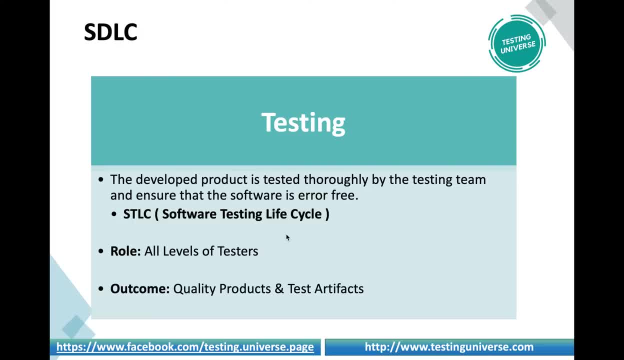 test managers- all those persons will be involved. underscore, then outcome quality product and test artifacts. so test artifacts means lot of documentation. documents will be, you know, generated in this particular software test, like cycle in the sense. test strategy will be there, test plan document will be there. 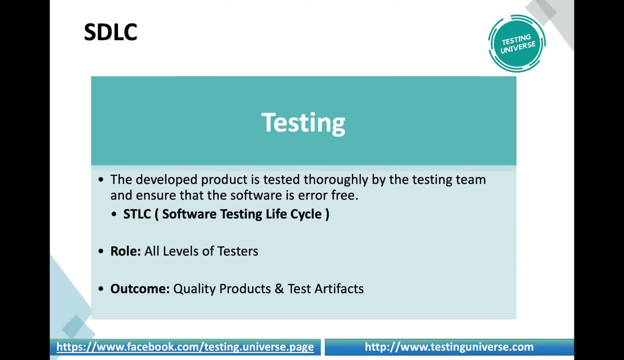 and you know, to test the product they will be having a systematic step-by-step test case will be there, right? so, and then the what: if you find some errors or bugs, that bug reports will be there. all those are called test artifacts. lot of documents will be the output of this. 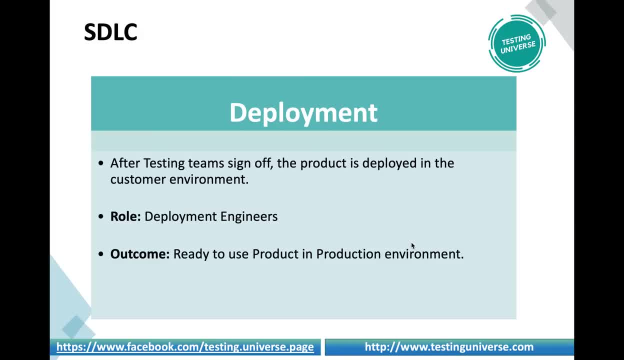 particular phase. once the testing is complete, right and test, once test management team gives a go-ahead for the product to you know, release to the customer, that particular product will be, you know, deployed or will be installed in the customer environment. in the development phase, development, there will be a development environment. in the testing phase, there will 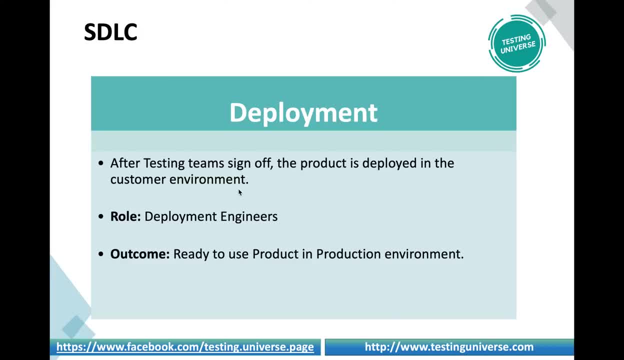 be a testing environment And the Customer environment will be the production environment. this will be the production environment. okay, so that is called deployment phase. once everything is done, after testing team sign off, the product is deployed or installed in the customer environment for the end user. 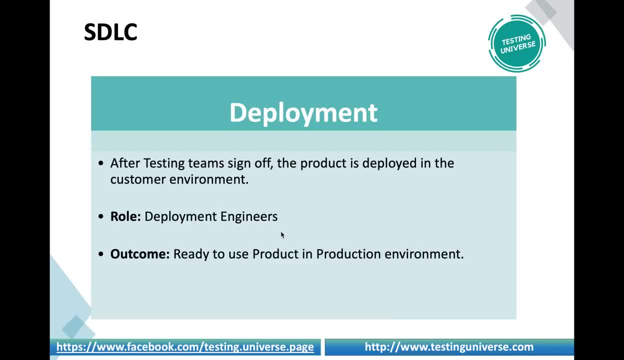 So who are all involved in this particular deployment phase? deployment engineers- there will be separate deployment engineers- will be there. they are going to deploy the product in the Customer environment. So what is the outcome of this phase? ready to use product in production environment. ready to use product in customer or production environment, the customer environment where we have deployed 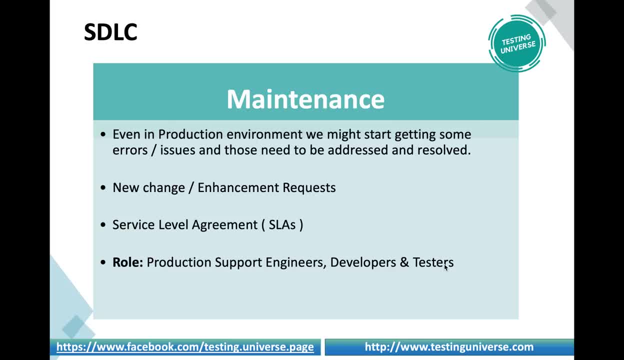 the software is called production environment. So the last phase is maintenance phase. right even in production environment we might start getting some errors or issues and those needs to be addressed and resolved. it is not that you know, after doing So much of testing and development and everything the end product will be, you know hundred percent. 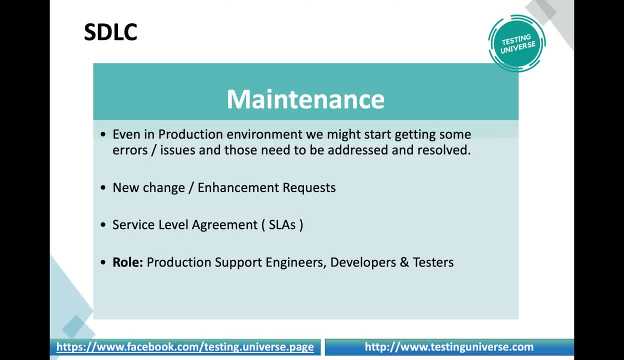 error free, that that will not never be the case, you know for, in any software development. So whatever errors you find in the production environment, those errors needs to be, you know, resolved or there will be, you know, some new change or enhancement request. So initially the customer for this inventory and billing software he might have told: okay. 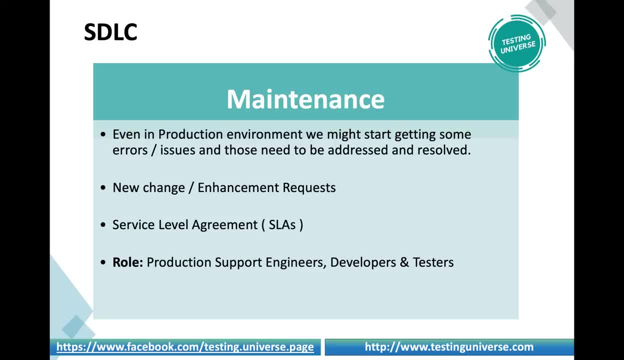 I have only one branch, but multiple. you know users will be there now after six months he will say, hey, I am, I am starting one more branch, the entire, you know, for that branch, the entire inventory and then billing and everything should be different. But the software, whatever you are going to, you know, give me, should be an integrated one. 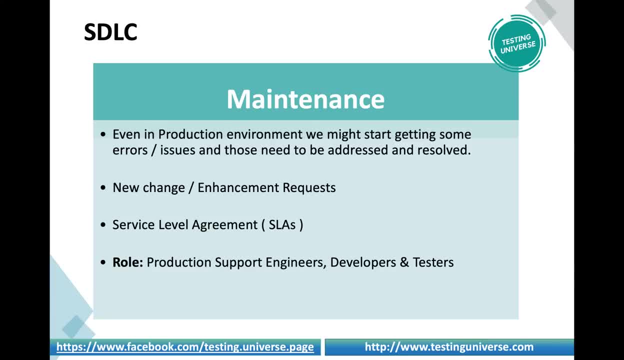 in the sense. So everything should be in one place. I should be able to see everything in my hand, in essence, all the reports and everything of that branch also. So for that, what do you need to do? this is a new, new change request or new. it is also. 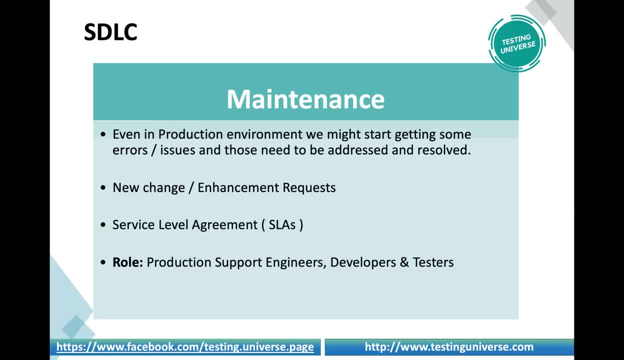 called as enhancement request. So you need to add one more module called branch module, where you need to create one branch. right there is a main branch and then branch two and then in that for that branch you need to start adding the users And then the stock and all those things. 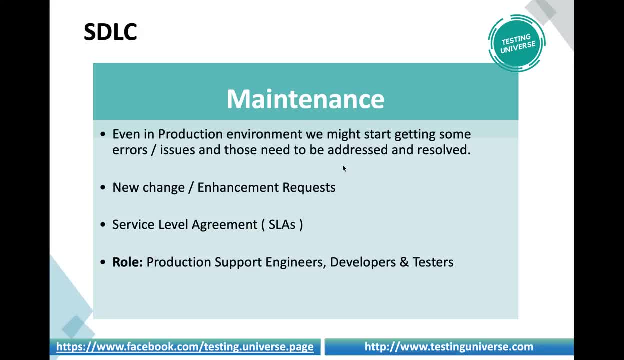 So these kind of requirements might also come in the maintenance phase. So how exactly this maintenance will be done? there will be a service level agreements between customer- you know, customer- as well as the development company, and then, based on those agreements, they are going to resolve the issues and then, if there are any new changes, that 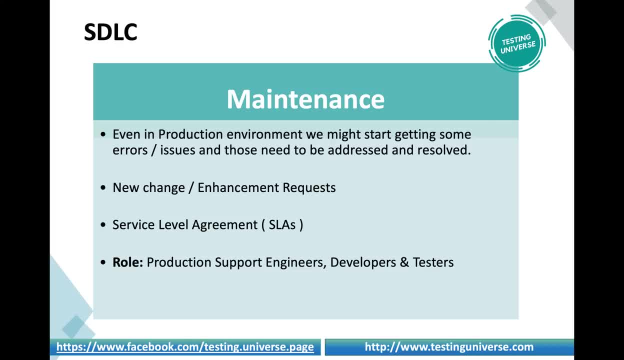 they will, they will agree that, okay, I will give you maintenance for two years for this amount. Anything I ask you should be able to do it, or that the agreements can be any time right. So in this particular maintenance phase, production support engineers, developers and investors. 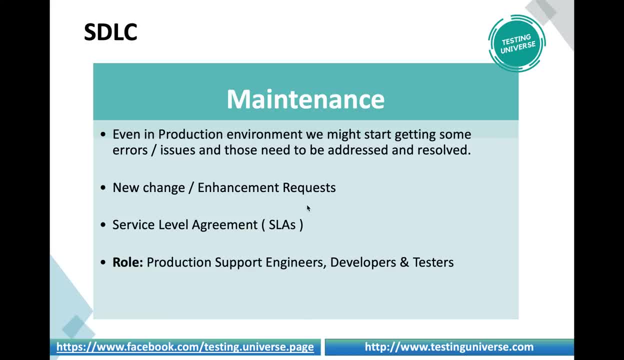 all these three people will be involved. if there are any new changes or requests, those changes needs to be, you know, first discussed with the production support engineers and then it will be passed to the developers. developers will develop those things and then it will be tested And then again it will be deployed and if there are any errors or issues, sometimes production. 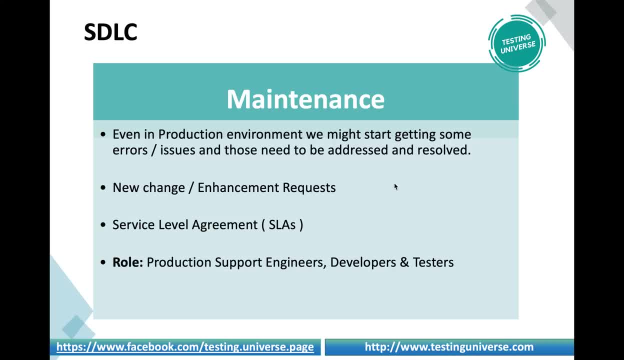 support engineers can also fix those issues or others. or if the customers have any queries related to any module or anything, will also be addressed by these production support engineers. So this is the maintenance phase in this is after completing the development. you need to know: maintain the software for. 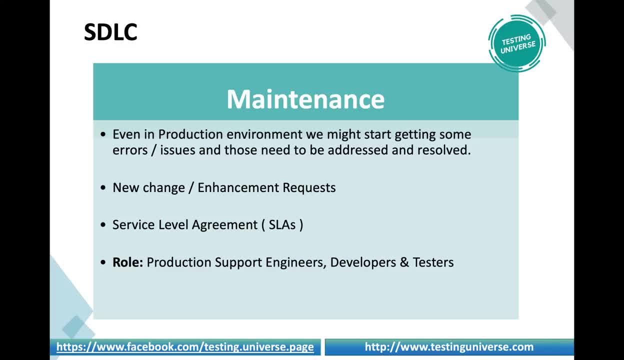 A number of years, for n number of years, because it is not that one year they will use, and you know, stop it, they might, you know, use it for many years with many, you know new requirements or many users or any any requirement come, for that matter, right. so it is also, you know, very, very important phase in software. 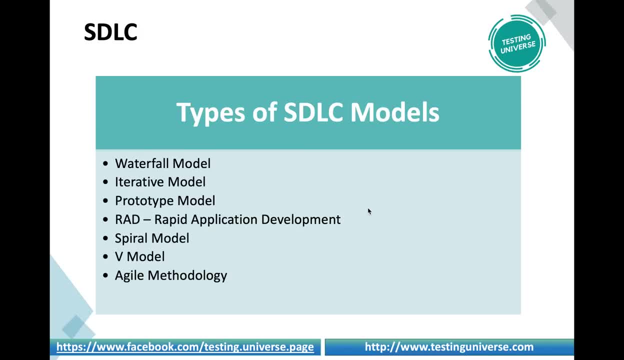 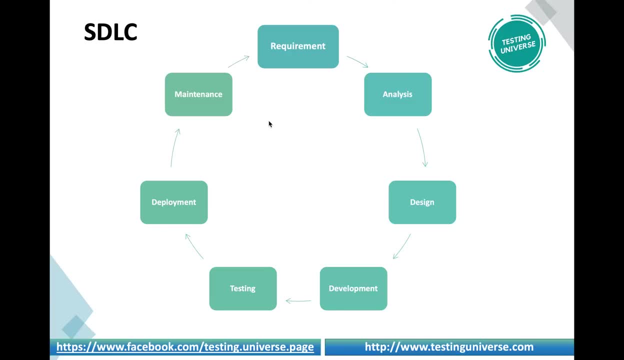 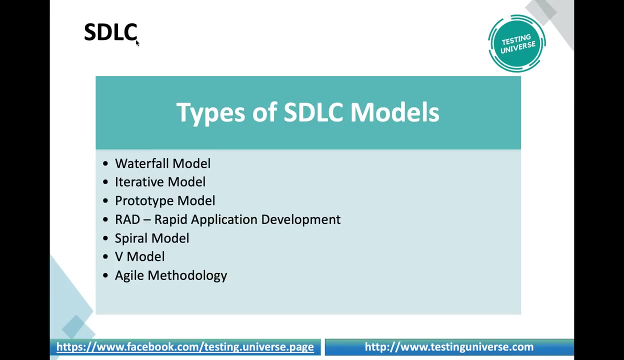 development life cycle. that's about the entire. you know the phases. whatever we have discussed here, all these different phases, right, and their detailed overview what, what happens in each and every phase, and then overall, will be involved in each and every phase of that particular software development life cycle. so in this particular software development life cycle we have different. 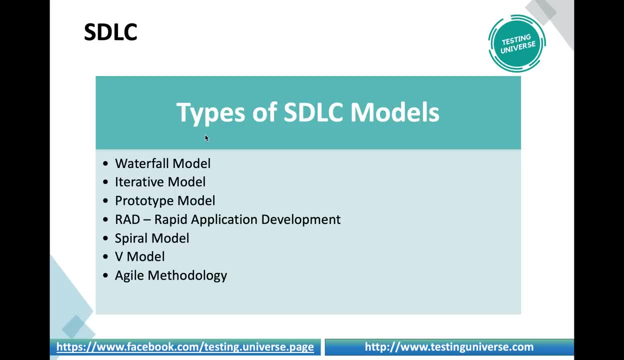 models. okay, so models are nothing but different approaches, right? for a small software, what needs to be the approach? for a big software, what needs to be the approach? or for a enterprise software, what needs to be the approach? right, so there are different. different, you know, approaches or models are there which are, you know, very standard and commonly used in the industry. 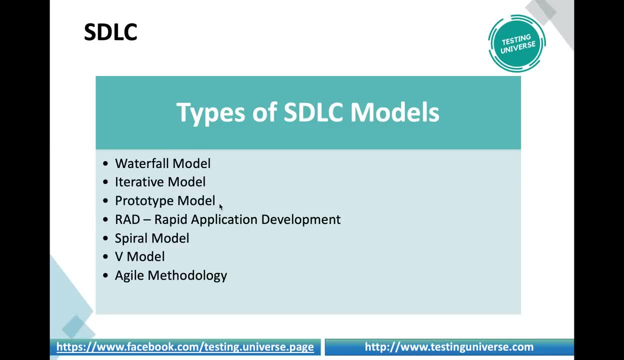 the first one is waterfall model, iterative model, prototype model, rapid application development, spiral model, v model and agile methodology. so these are all you know very, very important models which we have used. and then this is a traditional model, but agile methodology is the you know model which is used currently in the market. so we will. 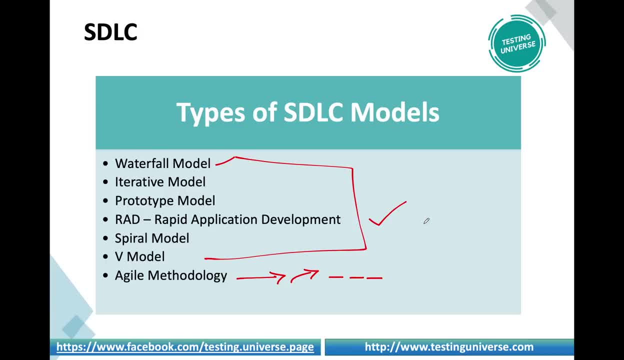 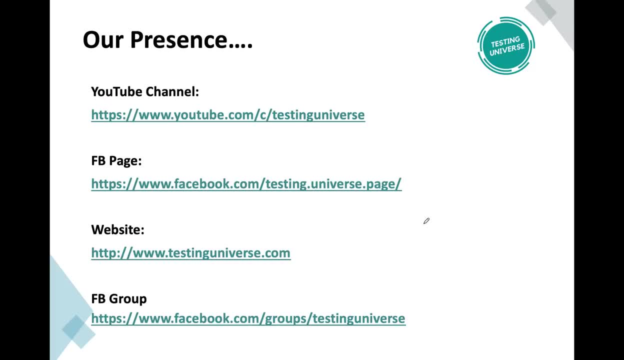 see all the important you know, sdlc models in our upcoming videos. so that's about software development life cycle. so if you like this video, i think i i have taken you know with a lot of examples. i have explained this software development life cycle because this is the 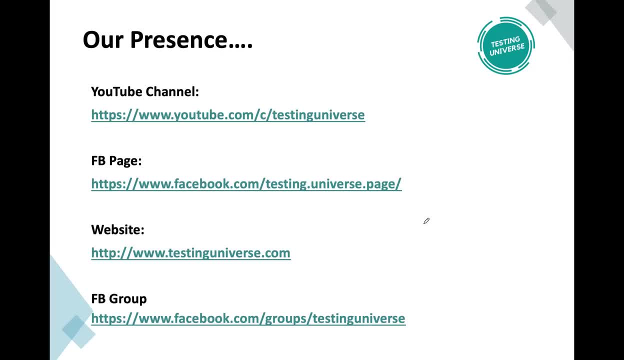 fundamental for any developer or any tester who wants to come to software industry. right, you need to know in detail about it. that's why i have taken, you know, this particular video a bit long, with a lot of examples and lot of explanation. if you like this video, please, you know, subscribe to. 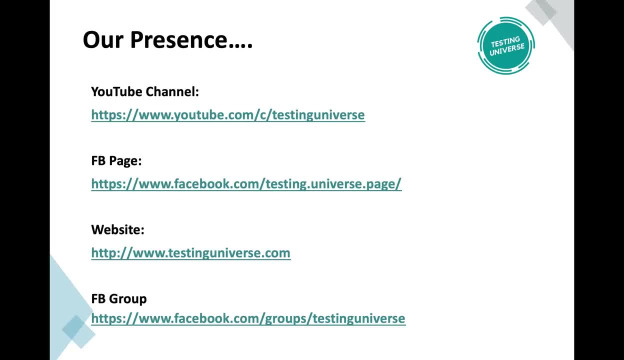 our channel as well, as we are present in all these different platforms, like we have a youtube channel, a facebook page, we have our own website and then we have facebook group. you can, you know, follow us on all these platforms. in each and every platform, we will come up with- uh, you know, a new stop stuff.